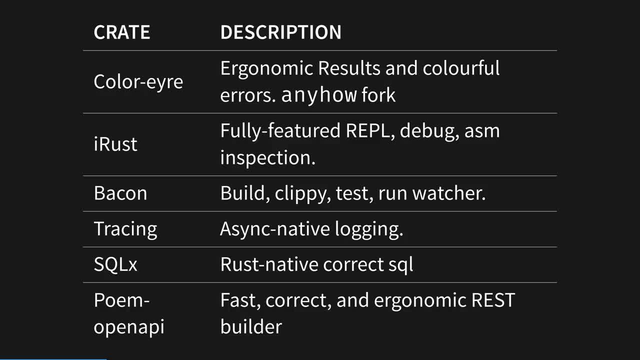 Luckily we have Rust. I have some crates that I use in nearly all my Rust projects. This feels like my own personal standard library. There are options for all of these. if you would prefer Anyhow to Air or EVCXR to iRust, You can't go wrong. 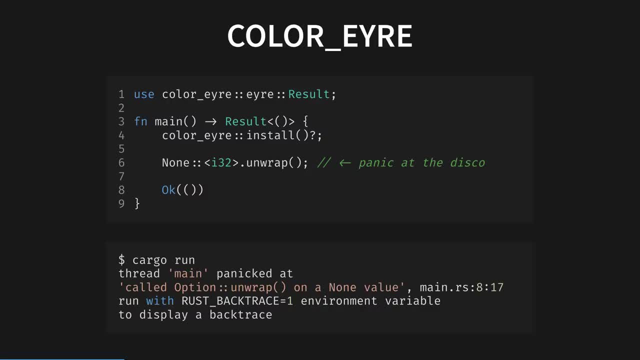 I'll explain some of them briefly. Air pronounced like the book Jane Air or the result variant, Result Air is a fork of the ubiquitous, Anyhow crate A trait object based error type for easy idiomatic error handling. but Air allows customisable error reports, which is exactly what Colour Air hooks into. 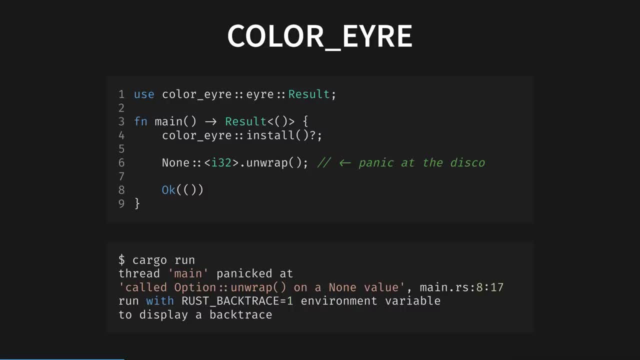 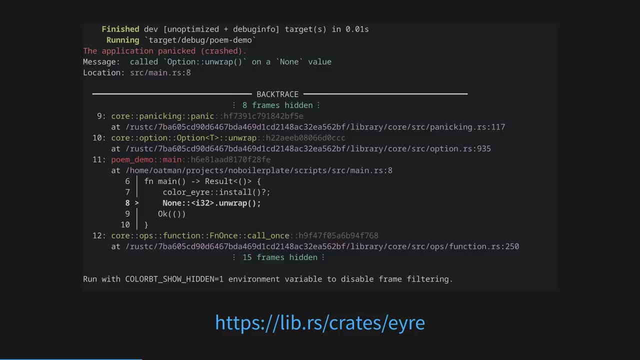 Install Colour Air as shown and enable the Rust backtrace environment variable and it turns this normal-looking Rust error, which is functional but boring, into a full-colour traceback. Runtime errors are dreadful in any language and with Rust they are. 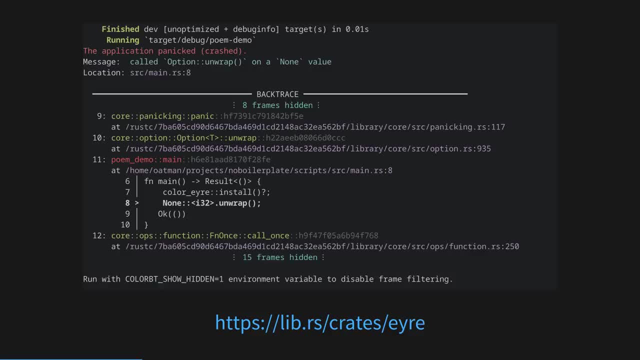 nearly always avoidable. However, there are cases where unrecoverable errors happen, and when they do, you will want Colour Air. The whole readme of Air is wonderful, by the way, and you should read the entirety of it. I love Bacon and if I'm coding, Rust Bacon is always open, running Clippy. 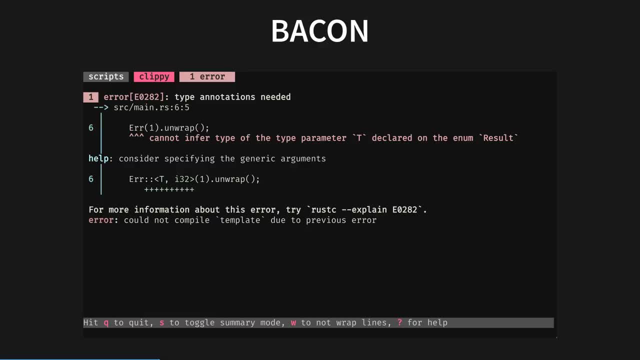 C after launch. even when I'm editing in an LSP editor, There's nothing clearer than Rust C's output, and when I'm coding, I need my conversation with the compiler to be as clear as possible. Tracing is Tokyo-native logging. Everything's in Tokyo: Web servers, HTTP request crates. 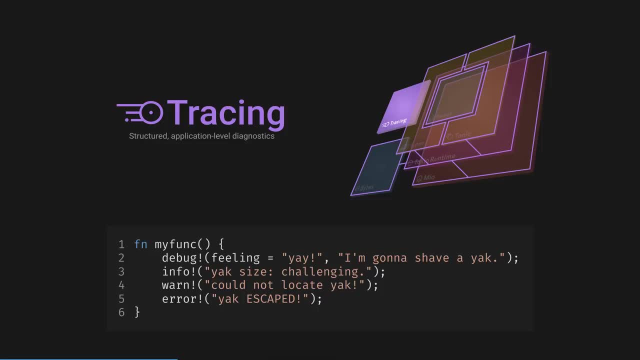 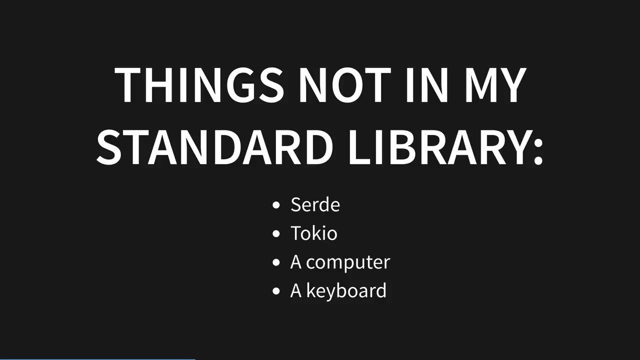 parallel processing libraries. You might as well start off with a logging handler that is great at async logging. My stack doesn't explicitly include Surdy or Tokyo. for the same reason, I won't be telling you to type with a keyboard or execute code with the CPU. It's. 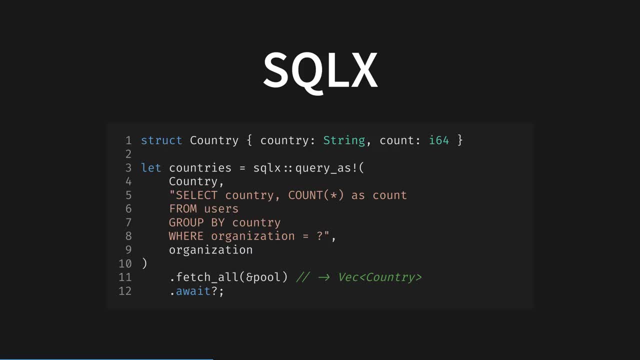 a prerequisite of using the other crates, so we don't need to go over them. I'll show you SQLX actually working when we build our API in a moment. but it is so alien you'll need to start processing this now. Here's the gist. SQLX allows the same structs you build the state of your program with. 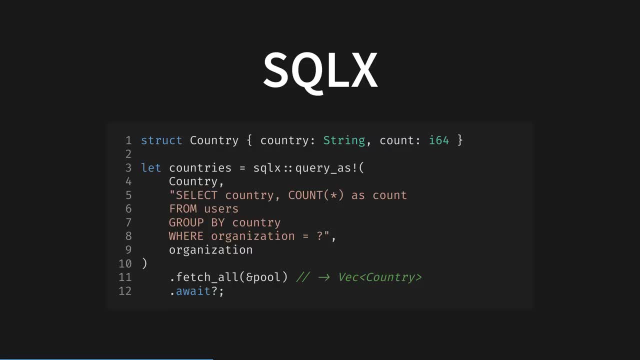 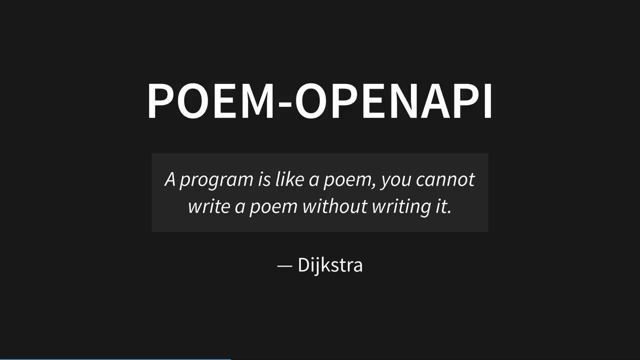 to validate your SQL queries at compile time. Got it? I'll pin my deep dive testing video if you would like to watch that too. Finally, the meat of the stack. A poem came to my attention in 2022 as I evaluated the Rust web framework landscape. There's a lot of really great options. 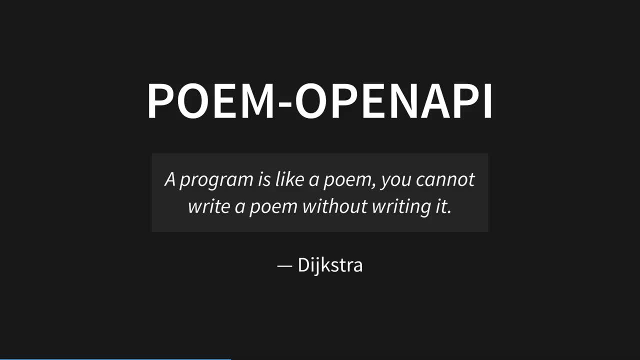 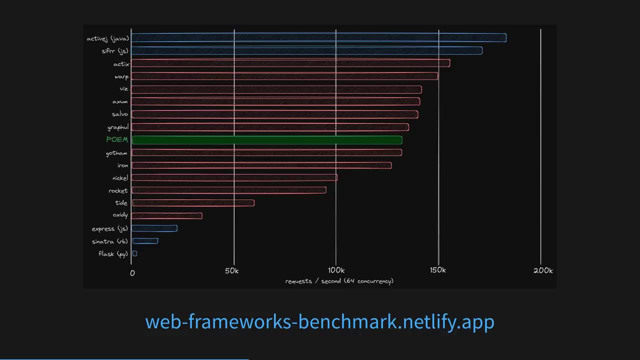 now I'm going to have to talk about benchmarks in this section, so I need everybody to be chill, okay. Okay, I have included all Rust frameworks alongside some fast and slow other frameworks. I discounted unpopular languages and frameworks. This included NIM, C++ and a lot of others that. 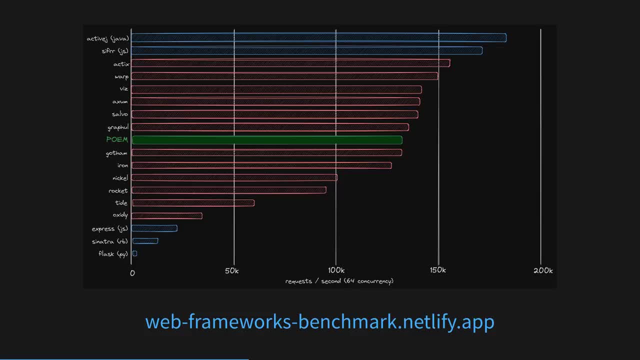 aren't relevant, You'll never persuade your team to use them, so you won't be using them. Popularity matters. That's why Rust is exciting. I used these synthetic benchmarks to get a feel for if any Rust frameworks were going to hold me back when scaling. And the answer is: 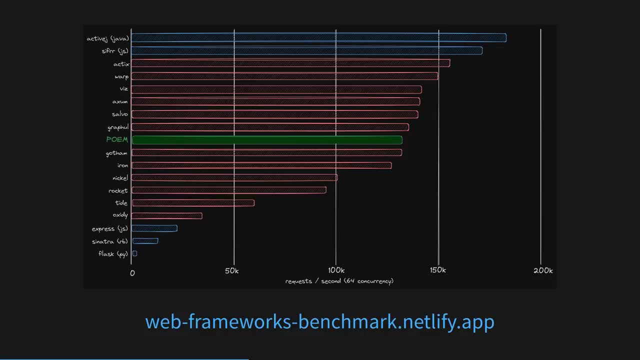 no, not really. As we all know, speed often isn't very important, but if you can have it, you might as well get it. To illustrate this, look at the bottom of the graph at our old friends Express, Sinatra and Flask. If this were a popularity graph instead of requests per second. 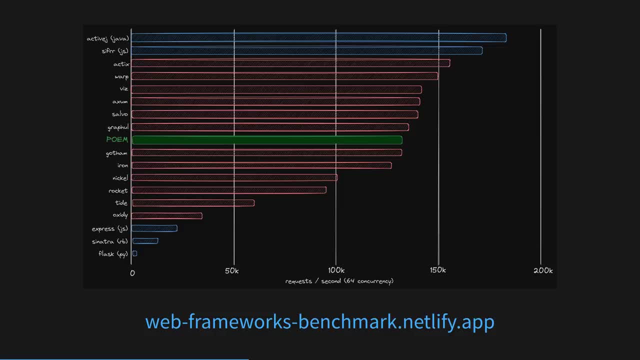 each of these mature frameworks would eclipse all above them. Our industry has decided that they are fast enough, and who am I to disagree? Looking at the top of the graph, to be fair and balanced, I have included the two fastest Java and JavaScript frameworks in the world. These are: 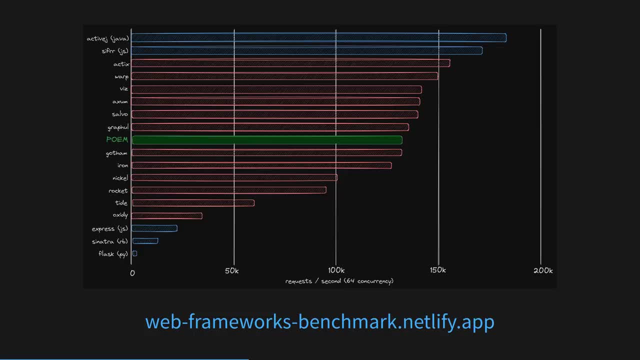 mostly native code tricks and are still only just edging out the Rust pack, despite both Java and JavaScript's literal trillions of dollars over decades in optimisation. Very interesting, So my search led me to this speedy part of the universe. Rust frameworks. that were all. 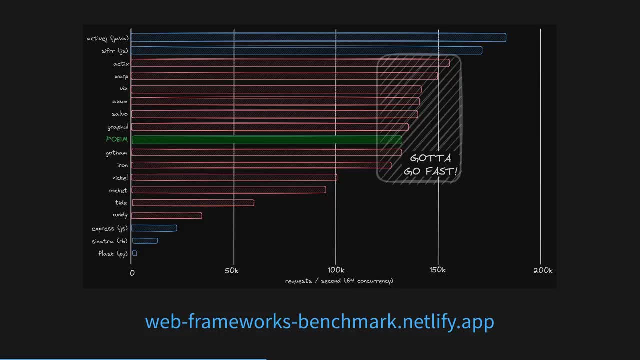 benchmarking at well over 100k, putting them amongst the fastest on the planet. After looking at them all, I fell in love with Poem, and specifically their first-party REST API plugin, Poem OpenAPI. Let's look at it. 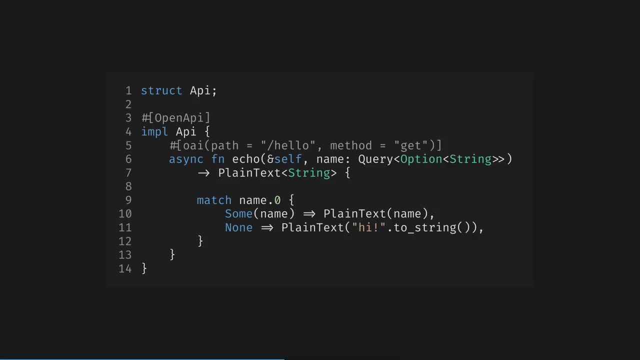 Here's a simple plaintext endpoint mounted at slash. hello, We have our top-level struct that we hang handler functions off. The OpenAPI macro surrounds this, adding lots of boilerplate that we don't care about. The OAI macro converts these simple functions into OpenAPI handlers. 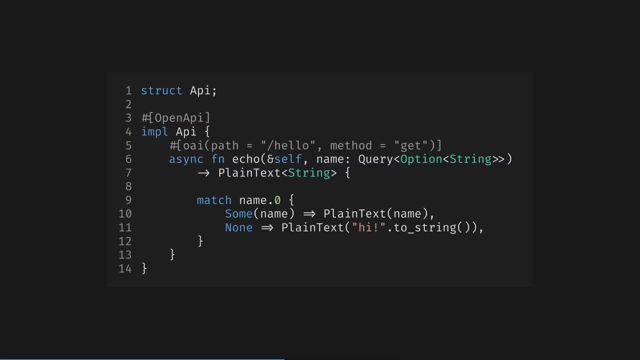 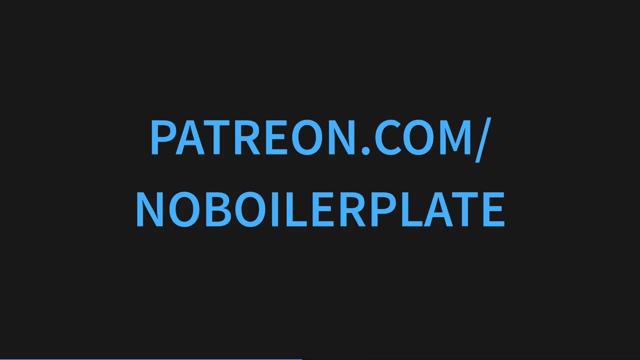 behind the scenes too. Then we have the handler functions with validated inputs, In this case just one echo handler, And the query type guarantees safe matching of query params at compile time. No ad- this episode thanks to my patrons, and before we build our API with Poem. I'll briefly. 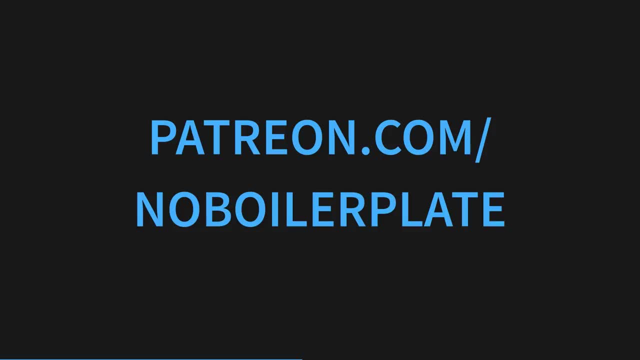 tell you about how this is possible. I have quit my day job and am now making videos and podcasts full-time, supported by my wonderful patrons and channel sponsors. Thank you everyone for watching and supporting me along this wild ride On my Patreon. there are various levels, but all get. 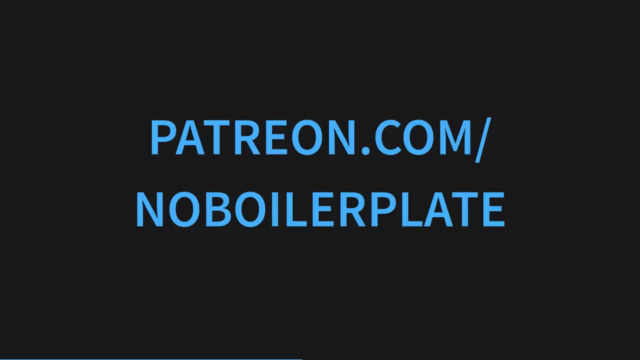 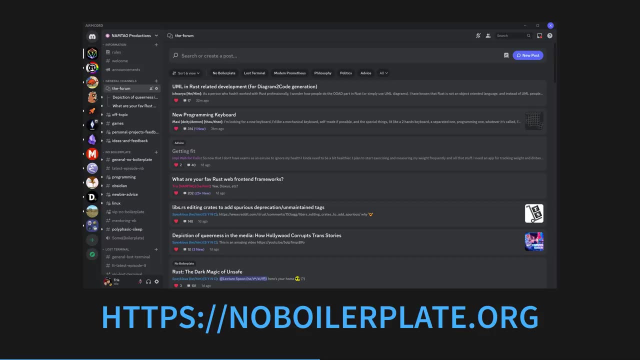 early ad-free and tracking-free videos and access to a private section of my Discord server. By the way, did you know? I run a huge Discord server- Over 2000 lovely people chatting about Rust, music, mental health and other cool stuff. Now that I'm doing production full-time. 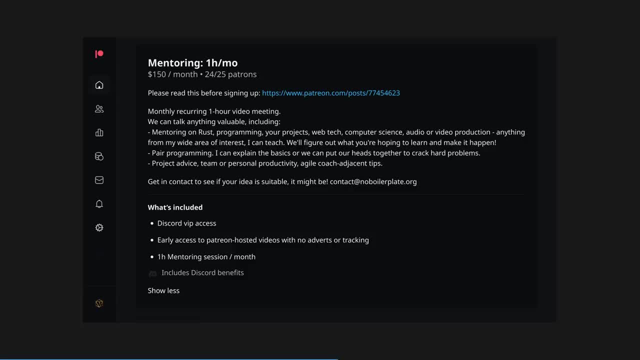 I have increased the number of slots on the new mentoring, Patreon and social media platforms. I can teach you anything I talk about on my channel- See the pinned announcement video for details. If it's fully booked, message me on Patreon or email me and I'll add you to the. 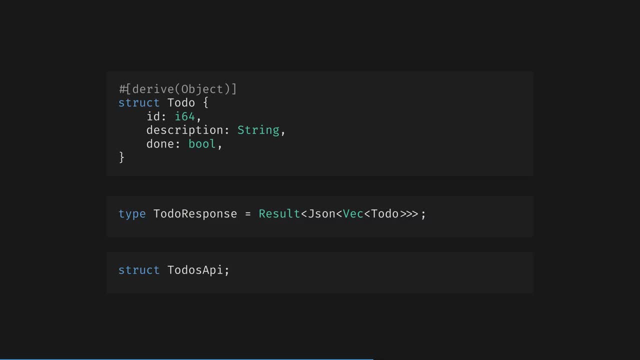 waiting list. Let's build First. as always, we start with the data model. These first two structs define both the database and API interface into our data. The third is a top-level Poem OpenAPI struct that we hang our API interface on. We'll see the implement blocks for this in a moment. 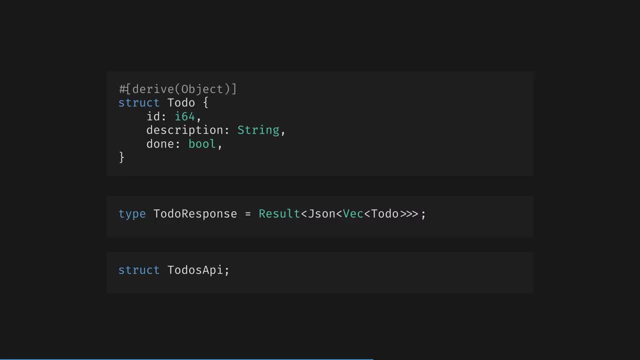 Binding your database and REST interface together at compile time allows us to have extreme confidence in our data integrity. This is a superpower: If you define your API in Rust structs, the compiler will stop you from breaking the contract with your API clients. Not only that. 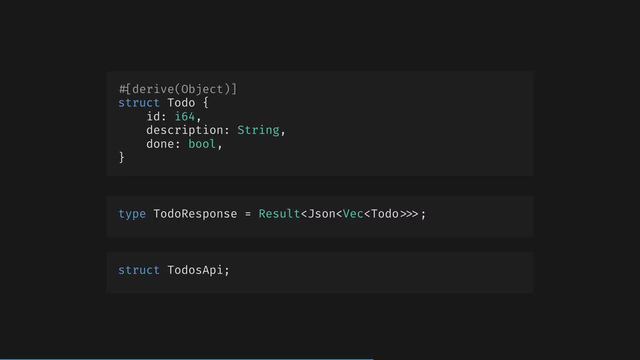 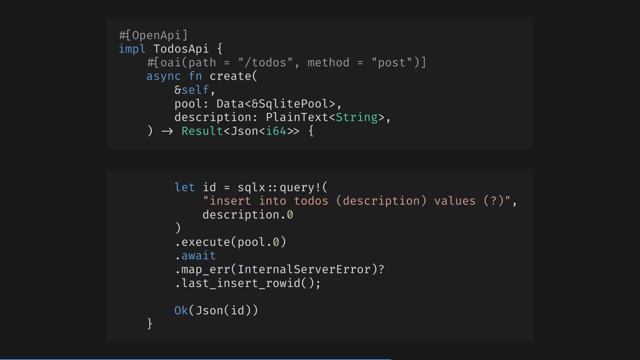 but if you don't see a PR where the structs change, your colleagues and collaborators haven't broken the contract either. Huge, Now we roll into the implement block for our To-Do's API struct. Our handler functions are defined here, with our database pool being. 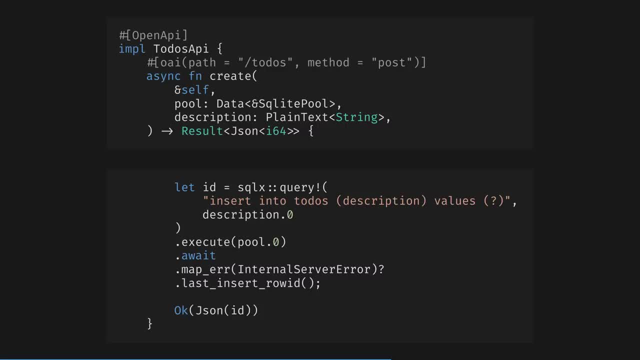 passed in as the first parameter and the post body as the second. This first function creates our To-Do's and handles a post to start the process. We can see that the first function is a post to Slash To-Do's. The return type is the integer ID returned by the database. 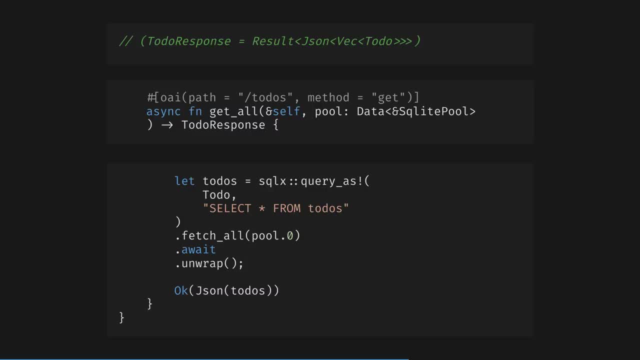 wrapped in JSON. Next we define the getAllHandler, also mounted at Slash To-Do's. The database pool is passed in here too, as it will be automatically on all our handler functions. It's passed in by the router, as we will see in a moment. You can see the return value. here is our To-Do response. 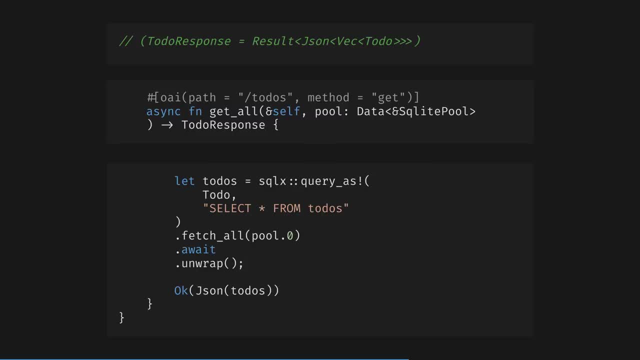 a vector of To-Do structs wrapped in JSON. Now we're using SQLX's compile time verified query to pull our To-Do's from the database. Note the parameter before the SQL query. That's our To-Do struct, the same that is used to define the items in our REST interface. 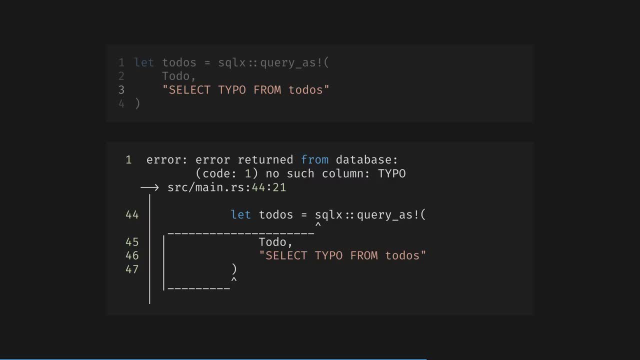 If I break the query, watch what happens. SQLX caught my incorrect SQL query by connecting to my local database, in this case SQLite, at compile time. This SQL error comes from the Rust compiler. SQLX taught the Rust compiler to understand how to connect to a database- Black magic right. 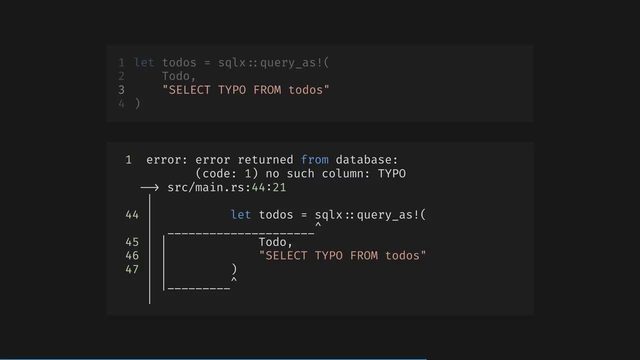 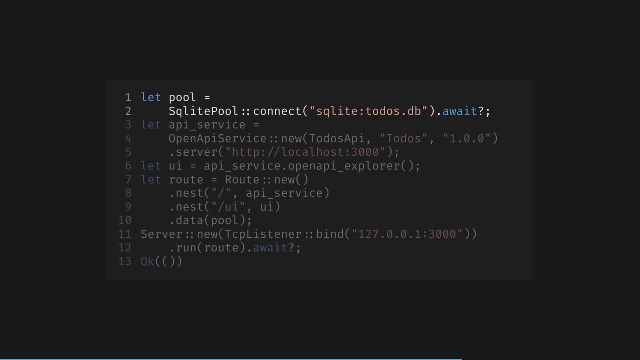 I have a video that explains what is happening here, called Rust's Witchcraft. Let's finish up with the poem. config in our main function. That's a bit much. Let's just focus on the function body. First, we set up our connection pool using SQLX. This is configurable but has sensible defaults. 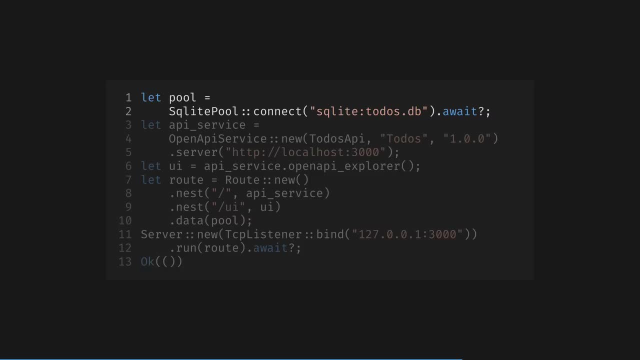 SQLX supports Postgres, SQLite, MySQL and MSSQL. If you have the choice, you should use Postgres. Next, we're building the poem OpenAPI service. Note: we've passed in our top-level To-Do's API struct. 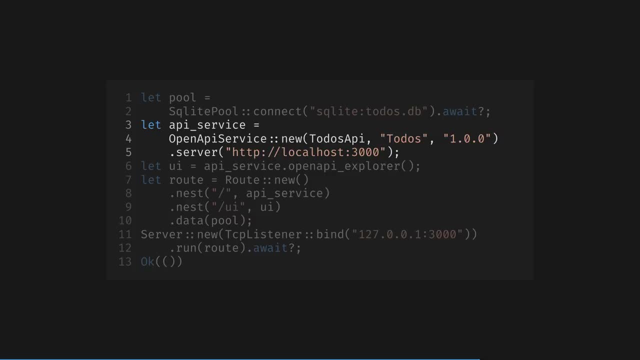 which has all of our handler functions implemented. Next is a friendly name for the API and a version number that is exposed to our API clients. We then build an instance of the OpenAPI explorer frontend. This is a built-in UI for poem OpenAPI and isn't the only one available. 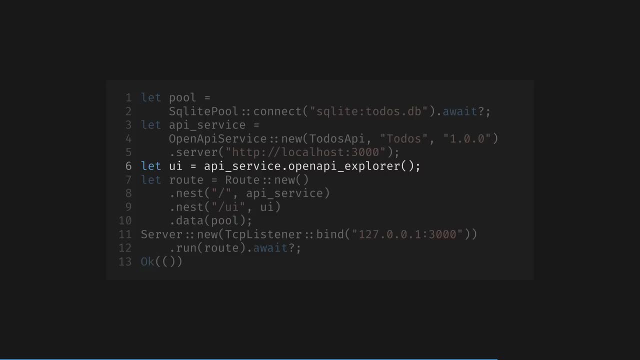 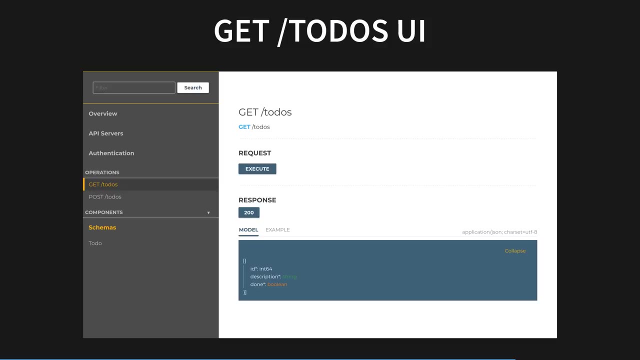 Poem also supports Swagger UI, RapiDoc and Redoc. Here's what our OpenAPI explorer looks like. Of the UI options bundled with poem, OpenAPI- OpenAPI explorer looks best to me. They're all built off the same OpenAPI spec that is built from your handler functions automatically. 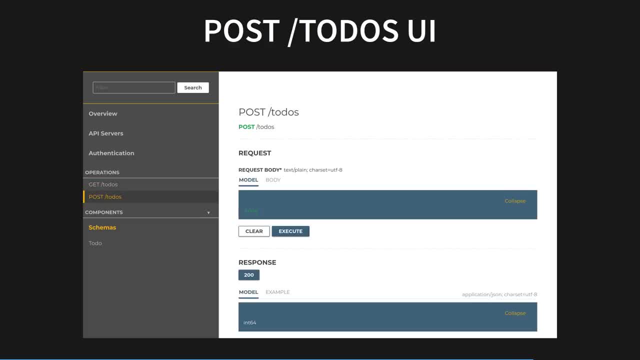 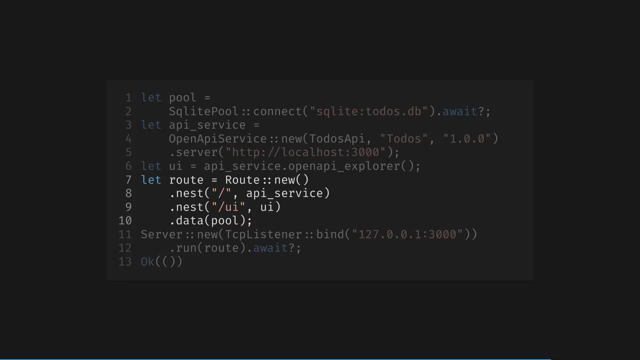 Note that this is all derived from your structs. Unlike in other languages, there is no need for separate API configuration here. Poem's router is very straightforward: The router is initialised using the builder pattern, adding routes with the nest method, the first parameter being where it is mounted. 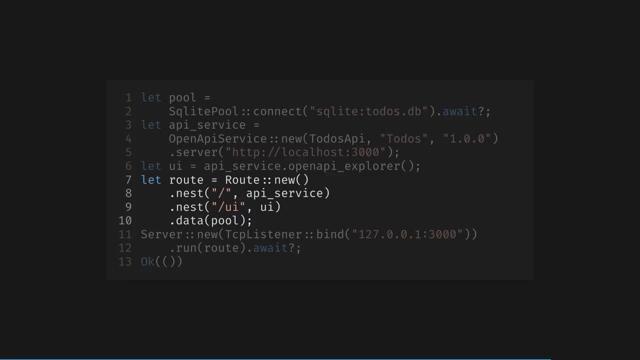 and the second the handler function of the API. This is the top-level organisational unit of your app. Think of large namespaces like login, user or search. You then build loosely coupled API structs that define their own URL namespaces under them. Lastly, the data method attaches state to the endpoint. This is how you 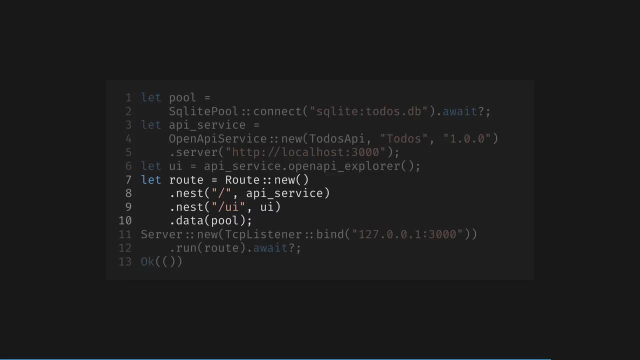 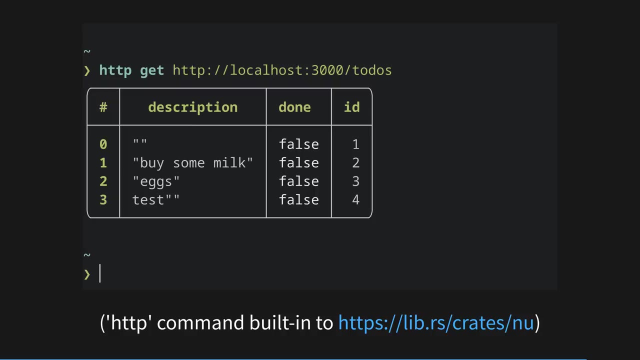 share state between your handler functions. The most common use of this pattern is to share in a database connection, as we are doing here. And finally, we start the poem server connecting the routes that we just defined. We did it A simple: post and get interface.